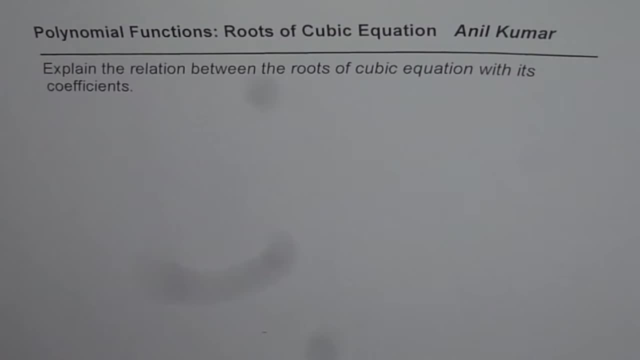 I am Anil Kumar and this is a very interesting video on polynomial functions. We will try to investigate roots of cubic equations. Question here is: explain the relation between the roots of cubic equations with its coefficients. What I am trying to say here is that a cubic equation 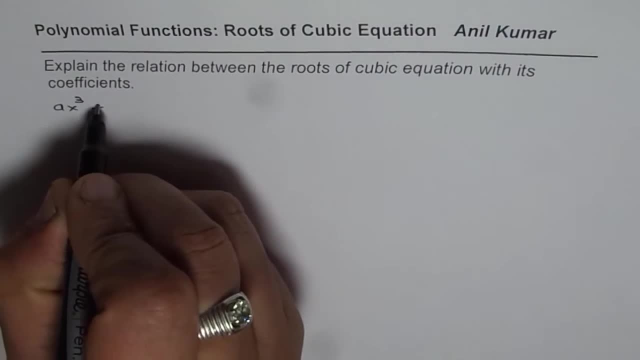 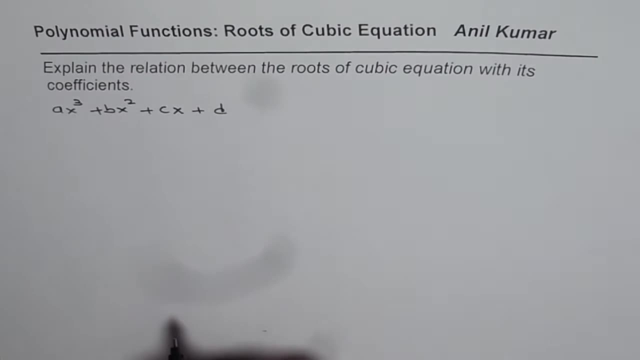 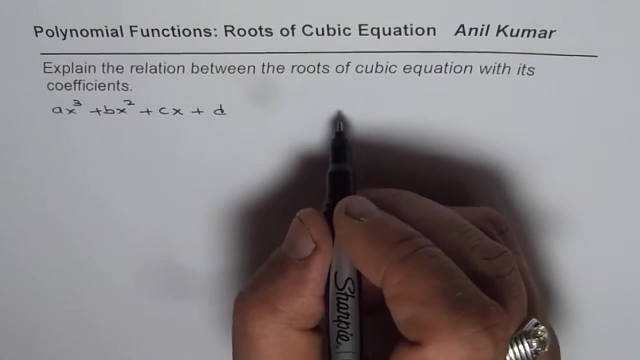 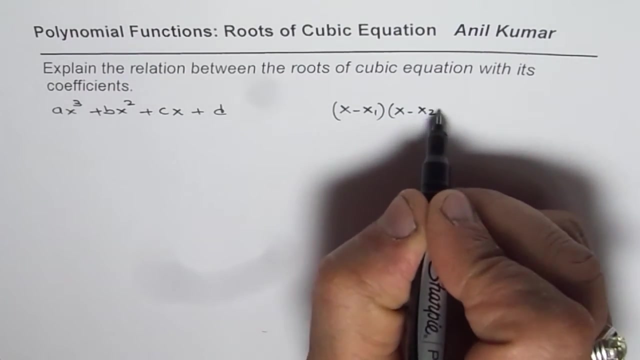 could be written as ax, cube plus bx, square plus cx plus t. So that is how we could write a cubic equation. Now we could also write a cubic equation in terms of its roots as x minus x1, times x minus x2, times x minus x3.. 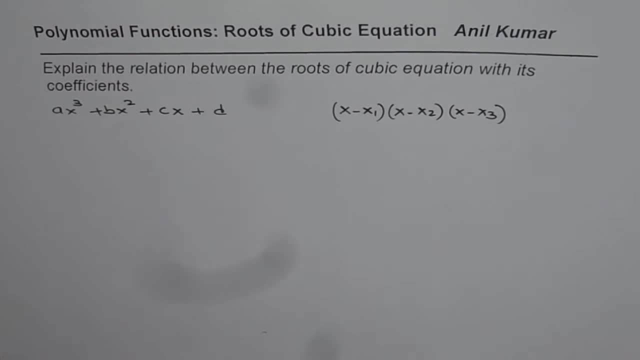 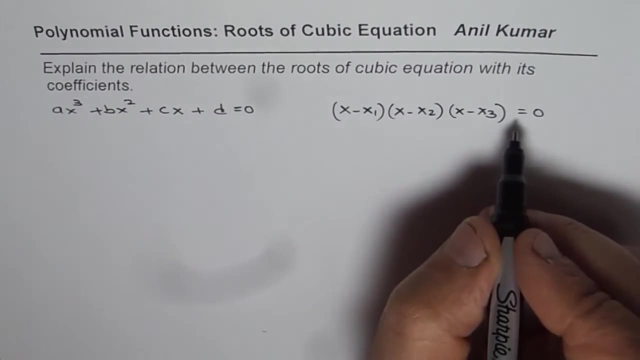 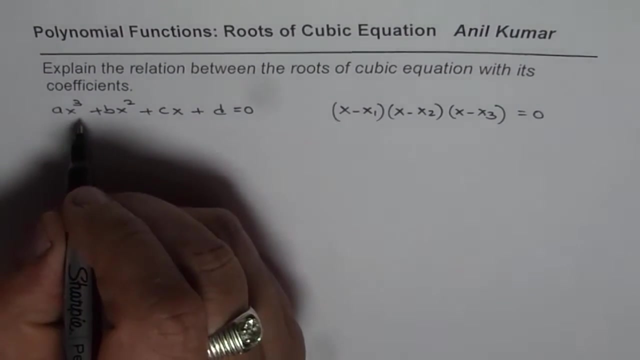 Cubic equation can happen in the following way: We have, at the most, three real roots. So all this equal to zero could be one form of equation which is in factored form, and here we have standard form of equation. So we have two different equations: This is standard form and that is factored form. 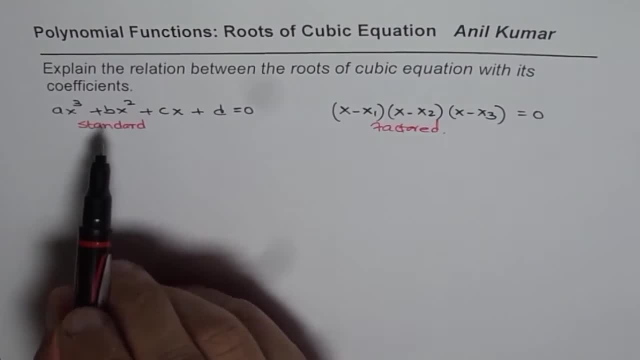 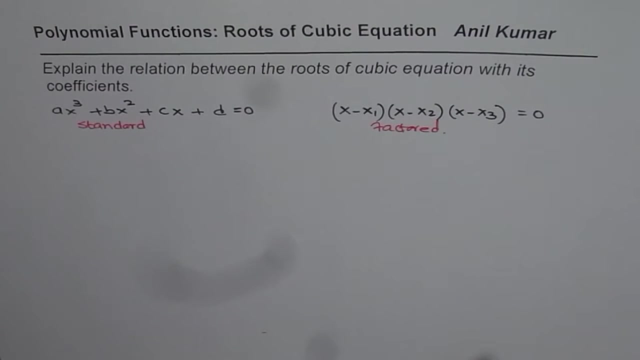 Now what are we going to investigate? We are going to investigate relationship between 2, x1, x1, x2, x3- the three possible roots with coefficients a, b, c and d. So that is what we are going to investigate in this particular video. So let us actually expand the factored. 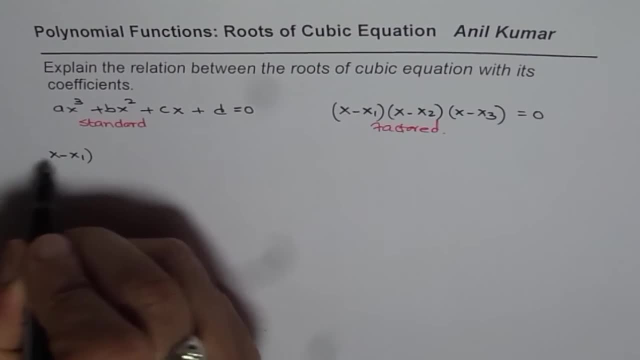 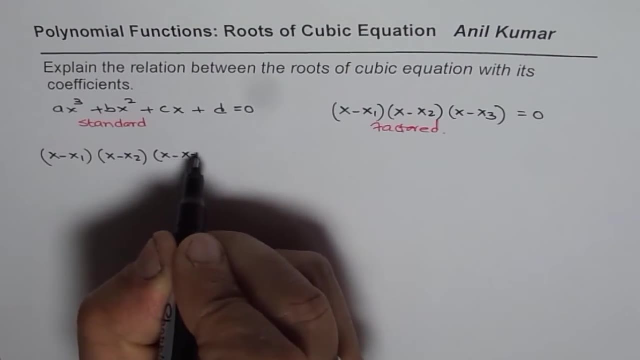 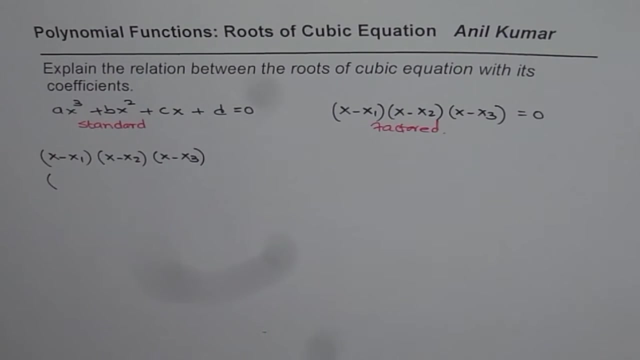 form and see what we get. So we have x minus x1 times x minus x2 times x minus x3.. Let us first multiply these two times. 1960, entrepreneur using analogue rock induce only half putt withoutб terms, so x times. so what we are doing now is we are multiplying these two first and then we'll. 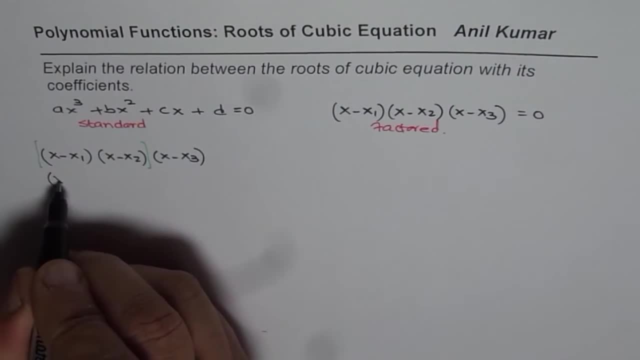 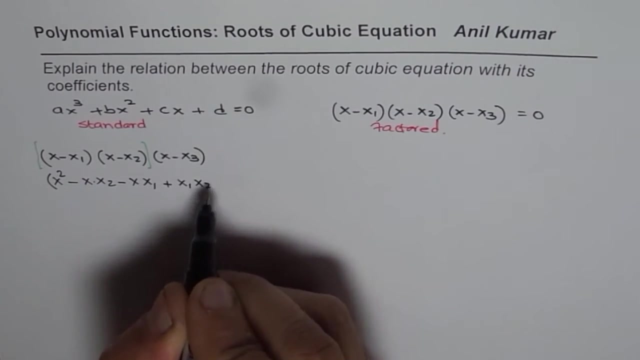 times that with x minus 3. so x times x is x squared. then we get minus x times x2, then minus x times x1, and when you multiply these two sign will be plus x1, x2. now with that, we'll multiply now x minus 3, right. so x times x squared will give us xq. now x with x will give us x squared. 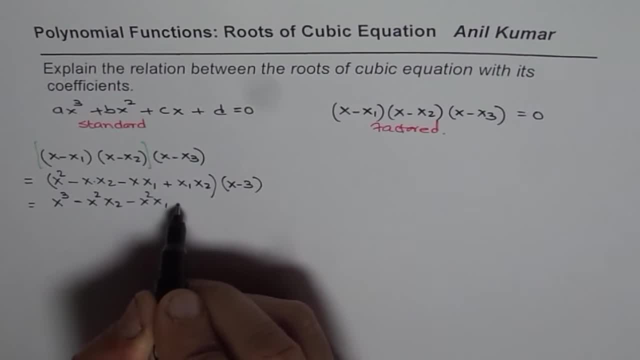 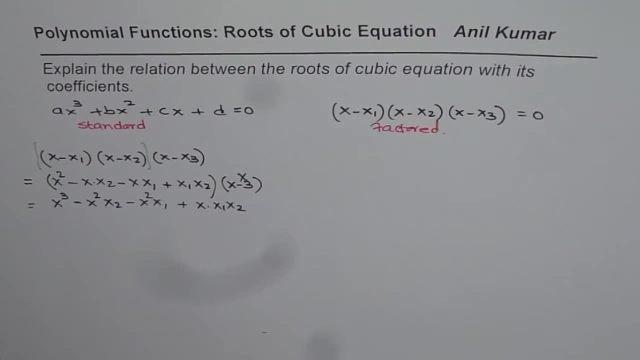 x2. then again x squared x1, plus x times x1- x2. i mean this is x3, right, okay, now let's multiply by x3 with a minus sign. so when you do that, you get minus x squared x3. x3 with x, we get minus x, x2, x3. minus minus makes it plus. then you get again plus x times x1- x3. 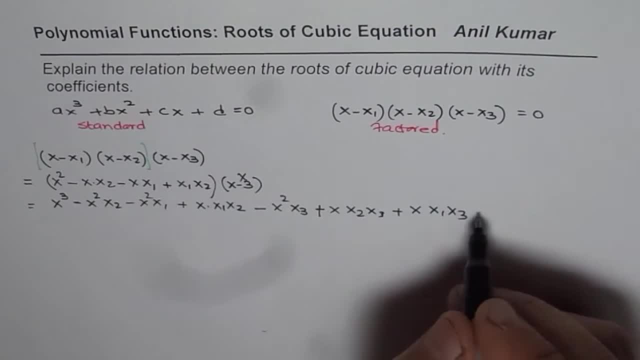 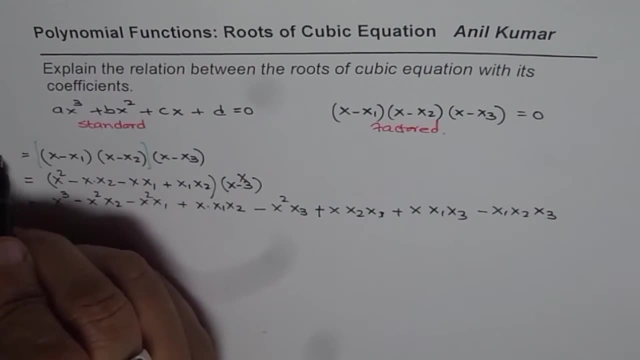 and then the last is minus x1, x2, x3. right now, all this is actually equal to zero, right? so that is how you get your factored form. now let us factor and write simplified form. so x squared, we have here. so for x, squared, we have. 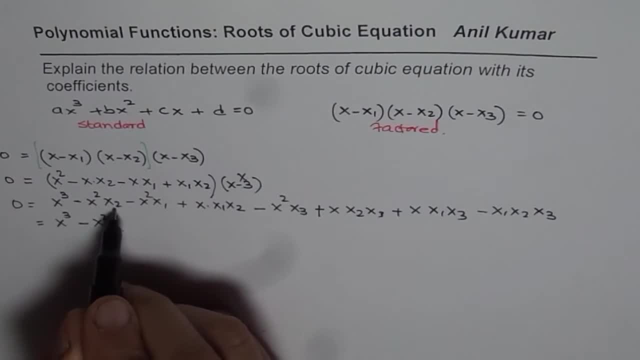 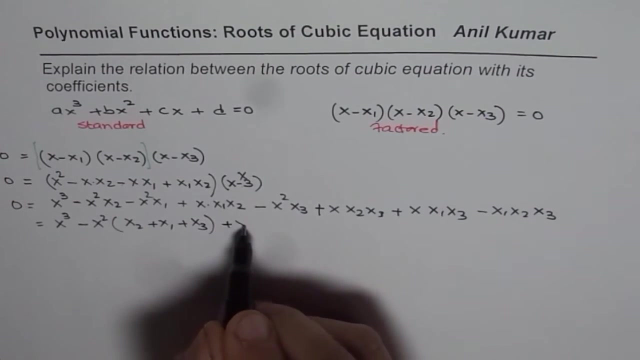 if i take minus x squared common, we get x2 plus x1, and with x squared we have x3 also. so three roots, sum of three roots. now let us see the coefficients for x. so it is plus x here, so we'll write plus x, and then we have x1, x2, and with x we have plus x2, x3. 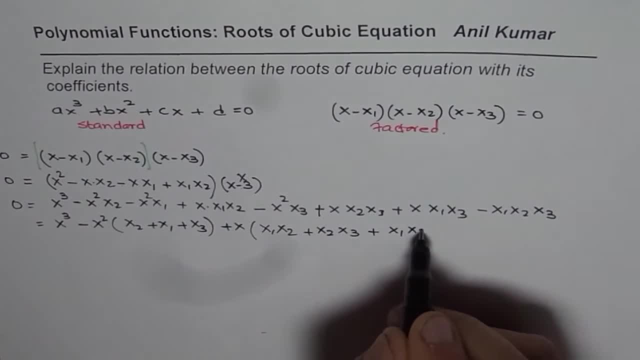 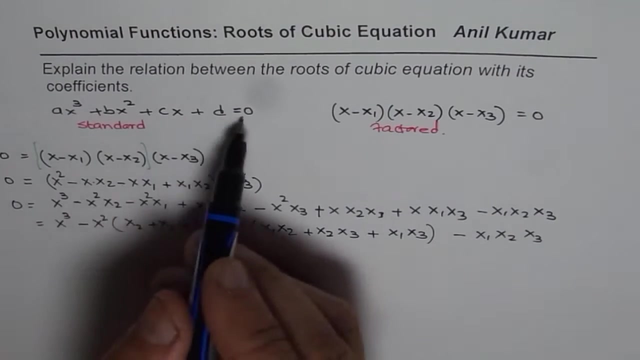 and with x we have plus x1, x3, right, and the last term here is minus x1, x2, x3. okay, now, if you are trying to relate these terms with the standard form, what do you notice? well, let me first rewrite the standard form: dividing by a right. so if i divide by a, then i get. 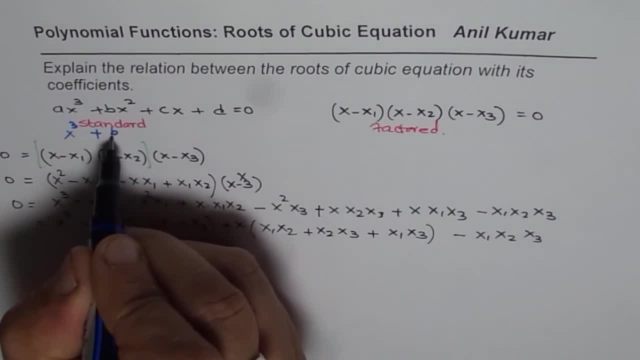 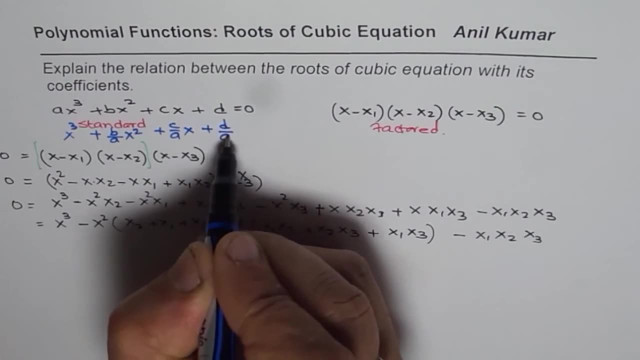 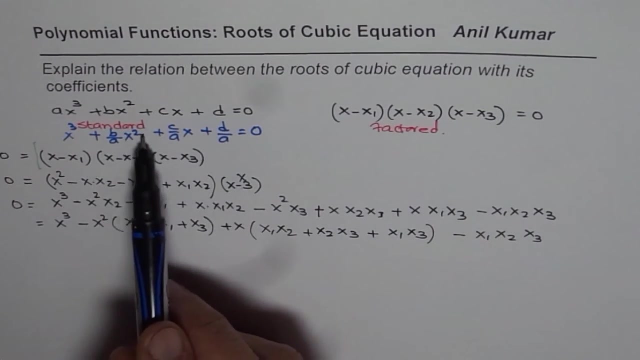 xq plus b over a, x square plus c over a, x plus d over a equals to zero, right? so if you compare, what we notice is that x square coefficient is b over a. here the coefficient is sum of roots x1, x2 and x3, right? so? so what you get here is b over a. that is negative, right? so we could write: